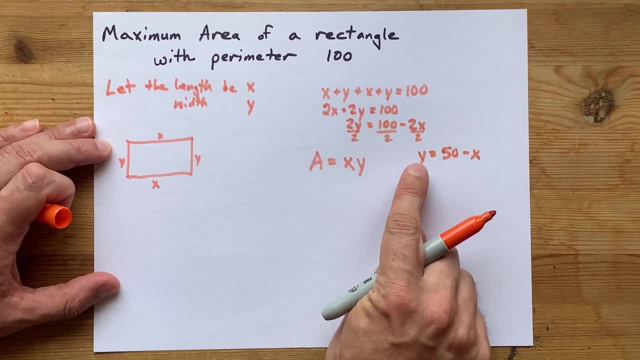 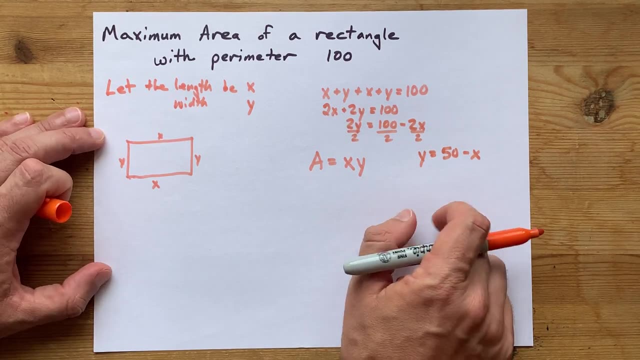 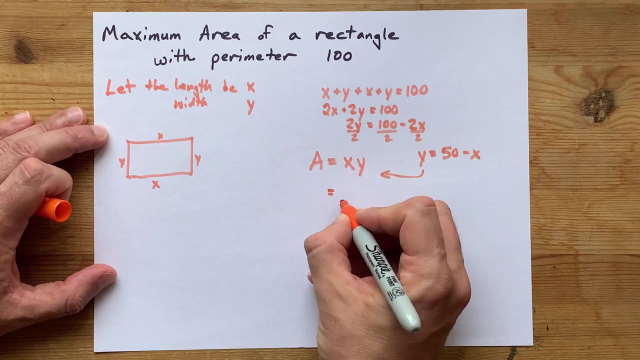 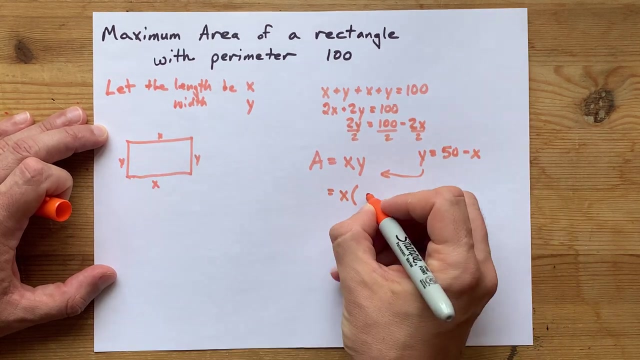 minus x. Now I've got an isolated version of y that's based only on x. What you can do from that point is substitute this into your area. equation: x times y is now x times whatever. y equals. y equals 50 minus x, So I'm going to put that there where y goes, Whenever I do a. 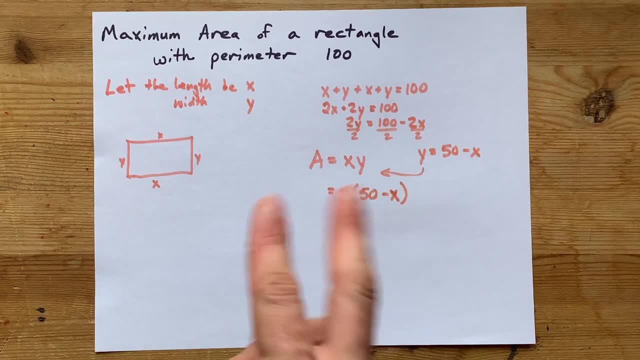 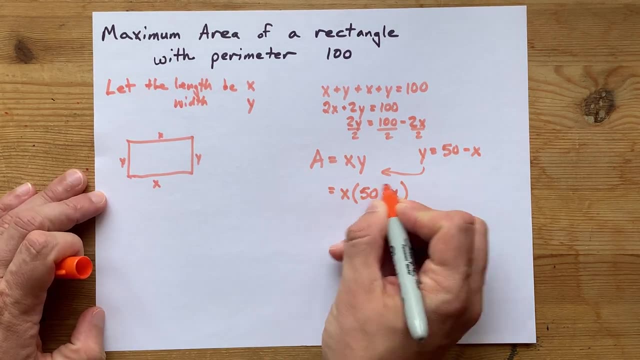 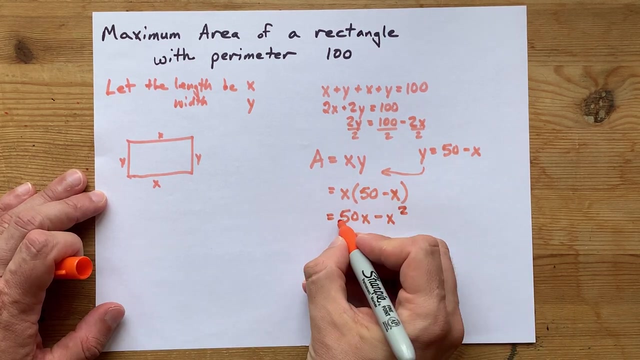 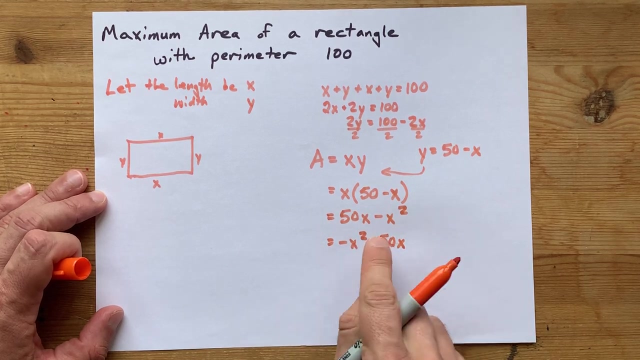 substitute. I like putting brackets around it. That helps me remember that this whole chunk is what y is. And now I'm actually going to multiply this out so you can see where we're going: 50x minus x squared, And if you want that in like parabola form, it's negative: x squared plus 50x, That's. 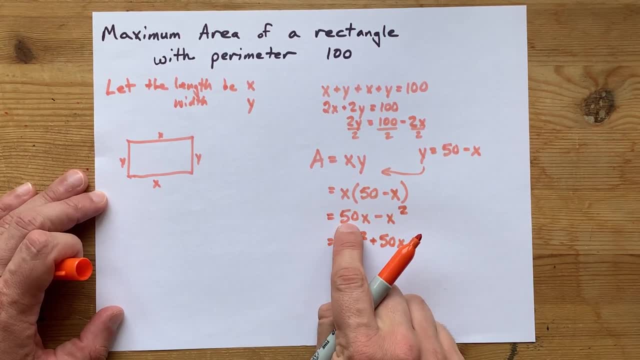 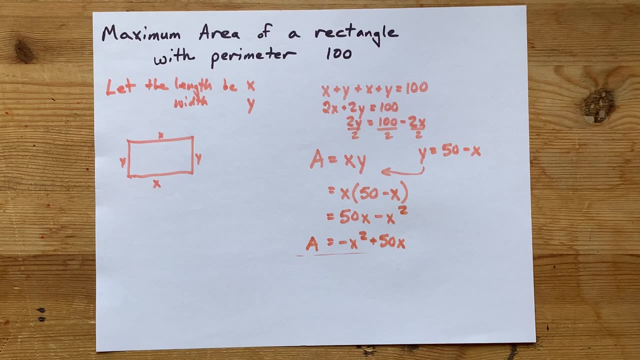 just me moving the negative x squared to the front and the positive 50x to the end. So this is the parabola we have to maximize. Now, the next thing I'm going to point out is that whenever you're asked for the maximum or minimum of a parabola, you're being asked to find the 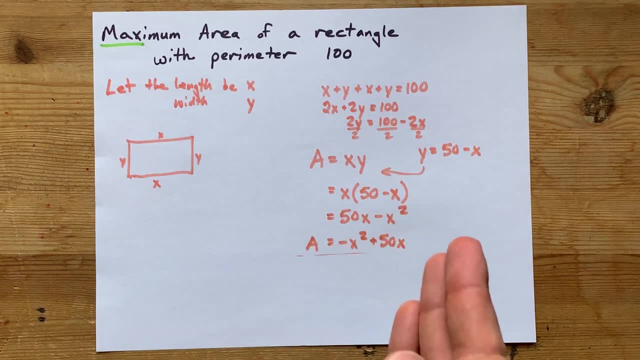 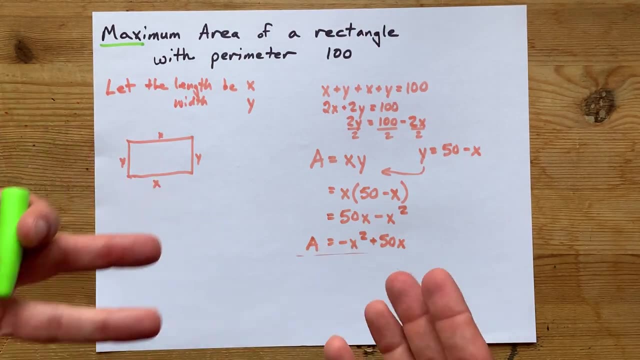 vertex. There's a whole bunch of ways you can actually find the vertex. You can do completing the square. There's shortcut formulas like negative b over 2a, if you've ever heard of those. But the way that I'm going to do it here is factoring. 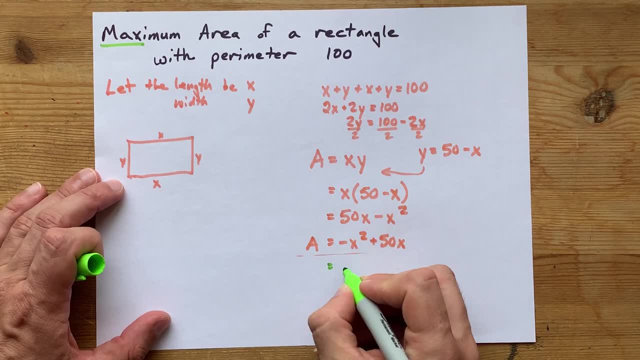 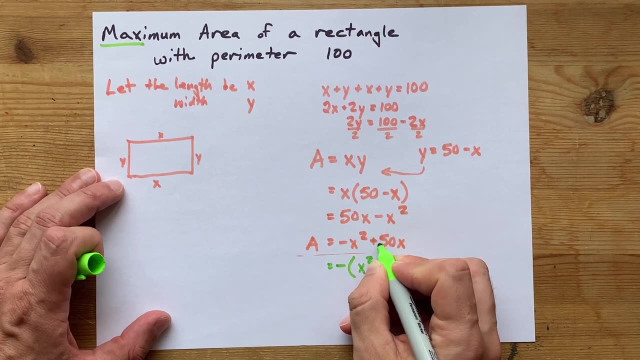 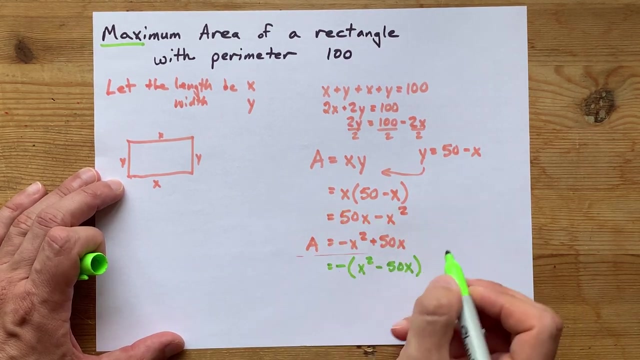 I'm going to factor the negative 1 out of the negative x squared here. Negative out of negative x squared is just x squared, and pulling negative out of positive 50x actually gives me 50.. Oh well, I'm actually going to factor an extra x out of this as well. I should have taken the. 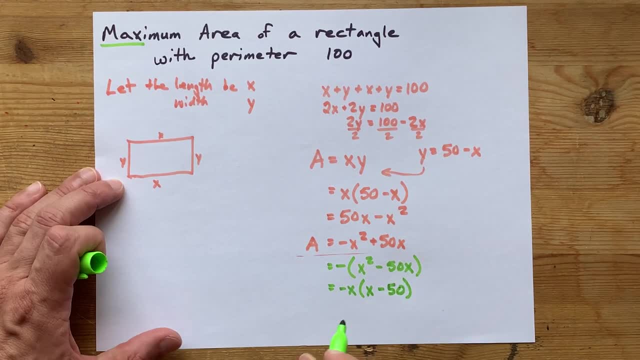 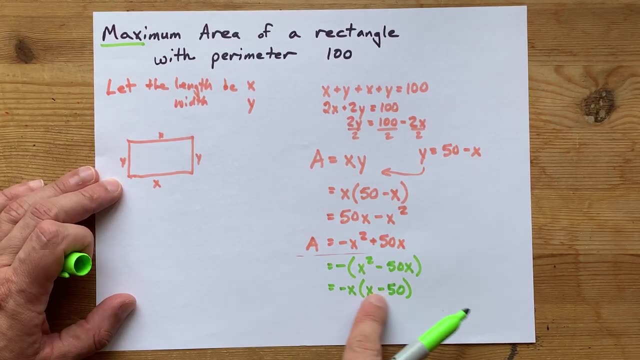 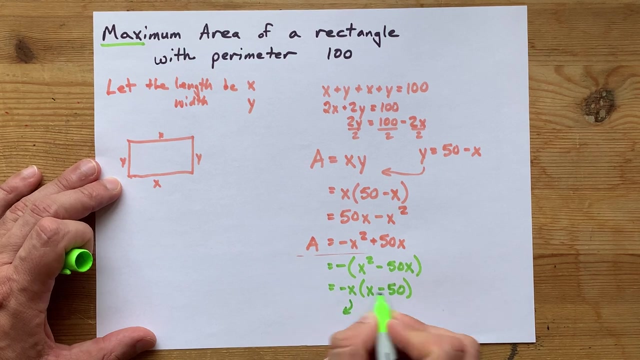 greatest common factor out of there before I did anything else. Now I'm going to feel a bit foolish because it looks like it was already factored here. We're basically already kind of there, except I factored in an extra negative there- The x-intercepts of this, and that's what you. 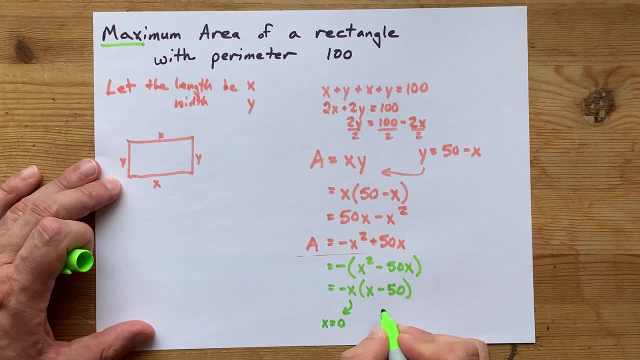 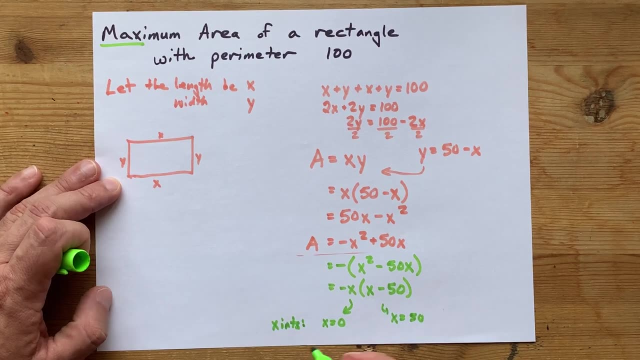 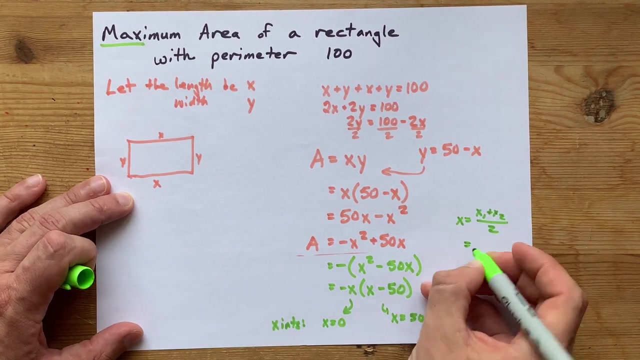 get out of. factored form after all, is that either x is 0 or x is 50.. Those are the x-intercepts. The axis of symmetry, or the place where the vertex is, is the average of those two. Some teachers will have you write: x equals x1 plus x2 over 2.. Again, you're just taking your. 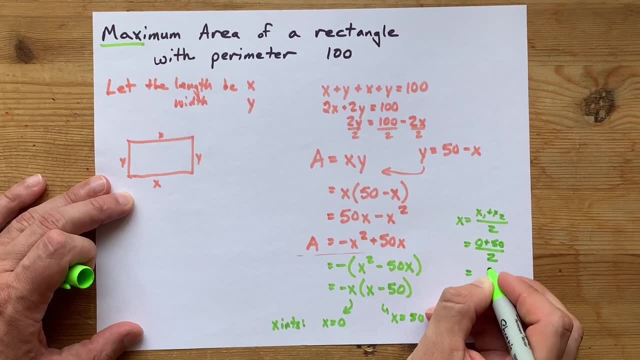 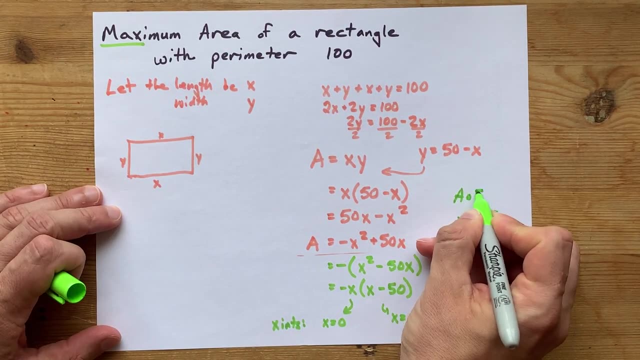 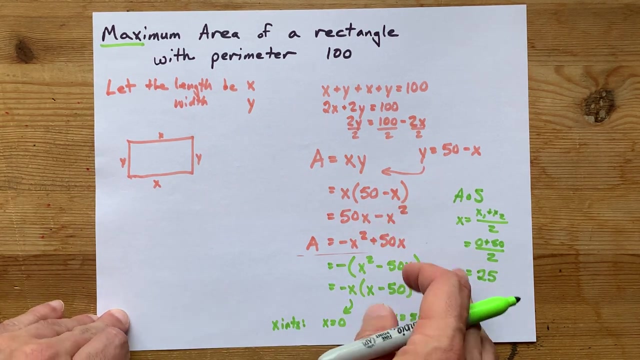 two x-intercepts. adding them up and dividing by 2, or averaging them, You get x equals 25.. That is the axis of symmetry for this parabola, the area, and so the maximum area itself corresponds to when x is 25.. Cool. 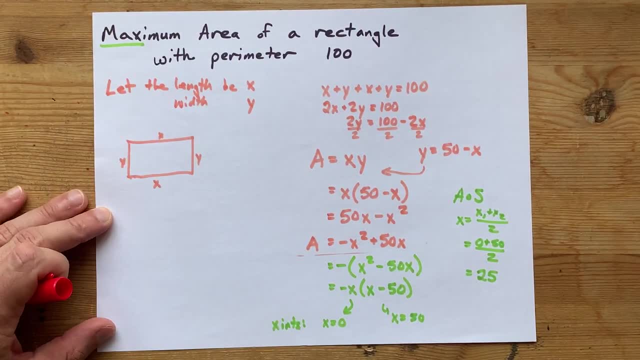 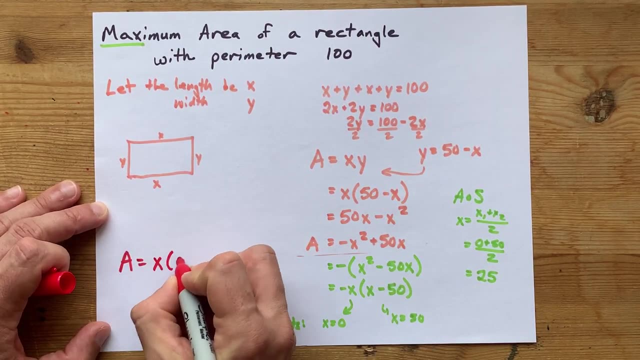 Now the question is: how do I get the maximum area of the x-intercept? The question itself is actually asking: what is the maximum area? Well, you can just take any of these expressions you had for area. I have x times 50 minus x, but I'm going to plug in 25. 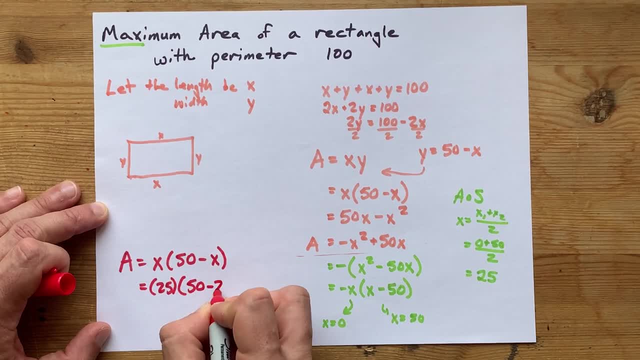 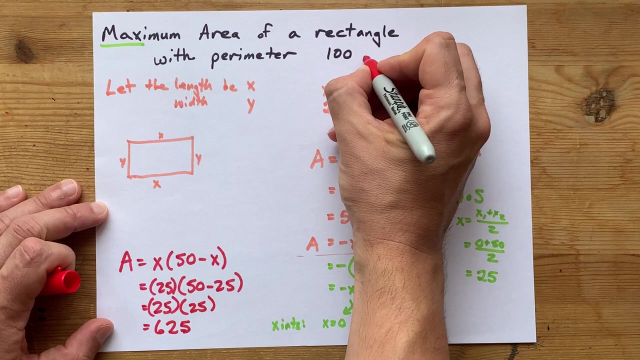 everywhere I see x. That's 25 times 50 minus 25.. That's 25 times oh well, 25 again and I get 625.. 5. Now I don't know what the units here were- inches or centimeters, or whatever- so I'm just 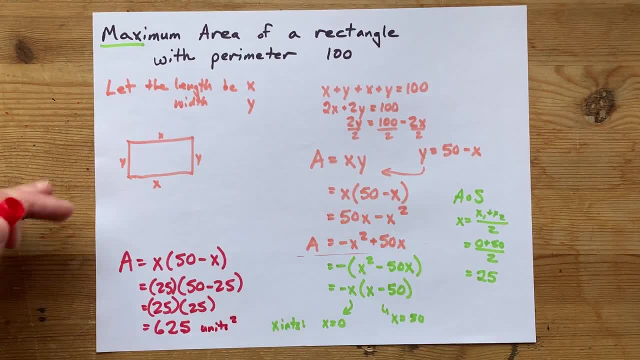 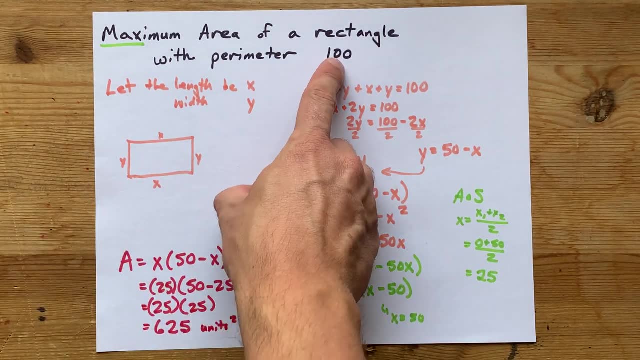 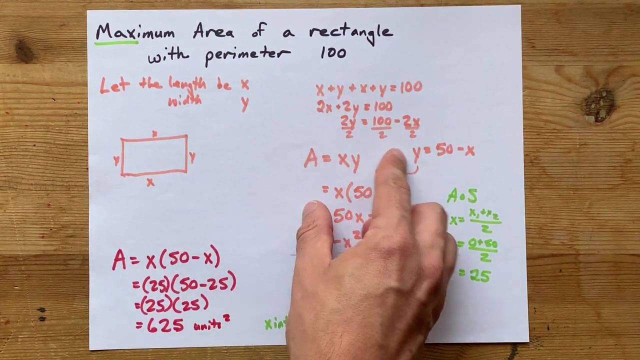 going to call this units squared. This question wasn't very clear about that. but the point is you're probably going to solve your question the exact same way, even if you don't have the same number there. Let x and y be your length and width. Get an expression for y in terms of x by. 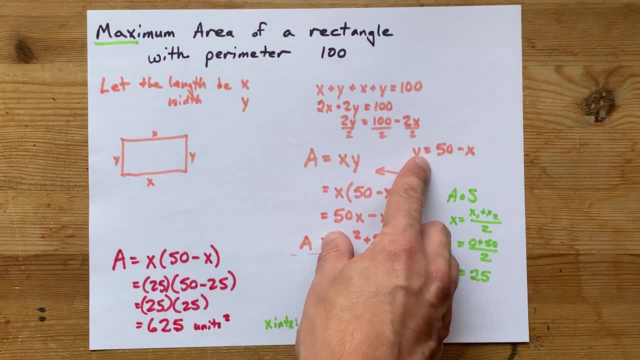 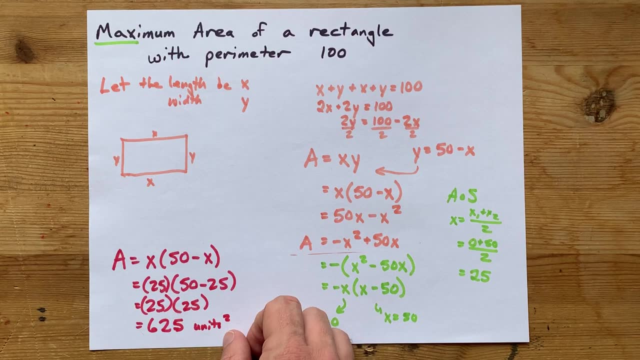 using the perimeter you were given. Use that isolated value for probably y in your area. expression: length times width. Get the vertex any way you know how: factoring vertex form, completing the square negative b over 2a, whatever- to get a value of x that represents. 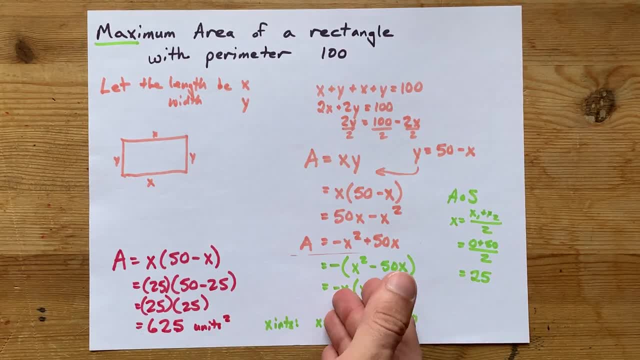 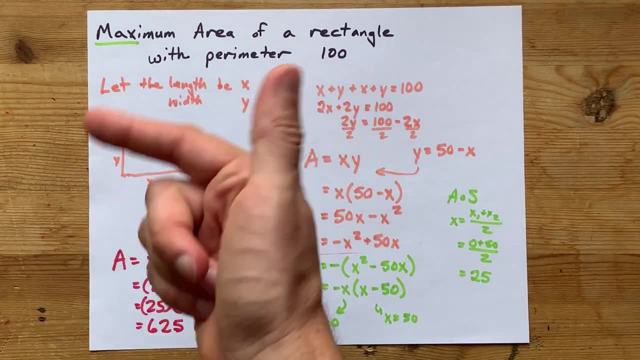 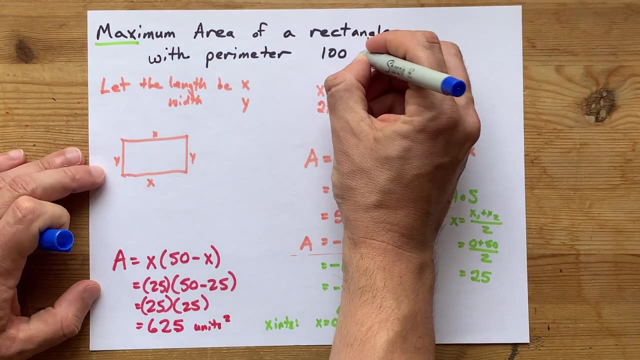 where the vertex is, Then you can plug that into the area formula to get the actual area. Now, if you're wondering what the shortcut is, the area of a rectangle is always going to be maximized for a square, So really all you have.